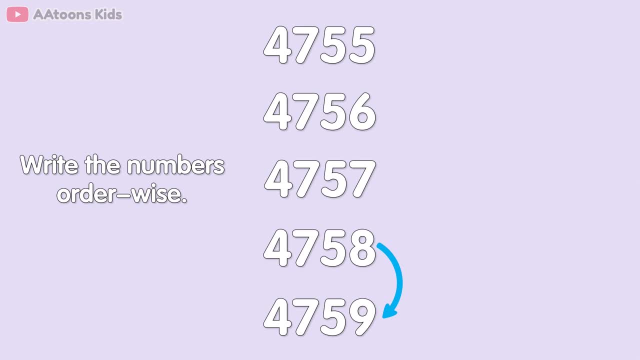 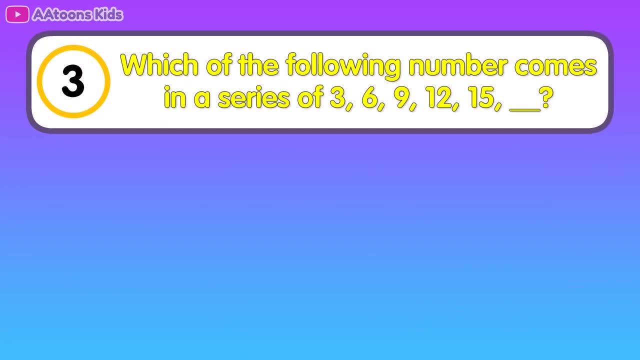 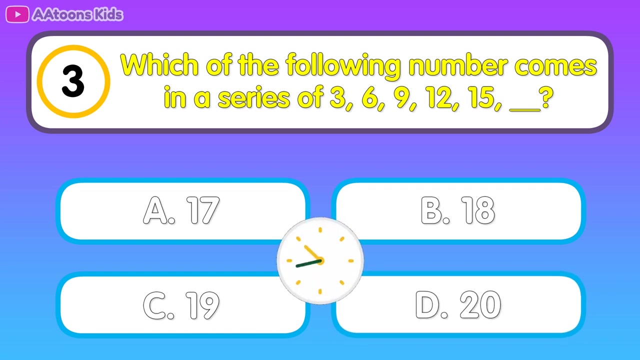 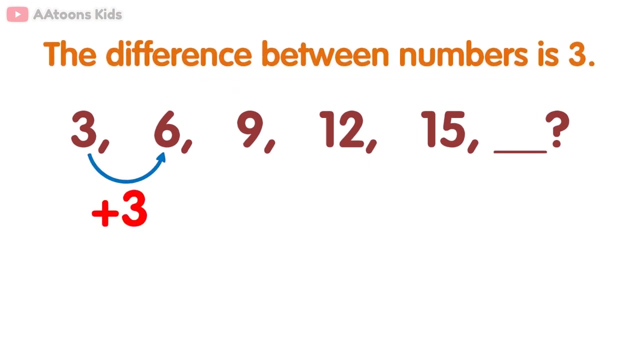 9 comes after 4,, 7,, 5,, 8.. Which of the following number comes in a series of 3,, 6,, 9,, 12,, 15? 18.. The difference between numbers is 3.. When 3 is added to 3 becomes 6.. 3 is added to 6 becomes 9.. 3 is added to 9 becomes 12.. 3 is added to 12 becomes 15.. 3 is added to 15 becomes 18.. So the answer is 18.. 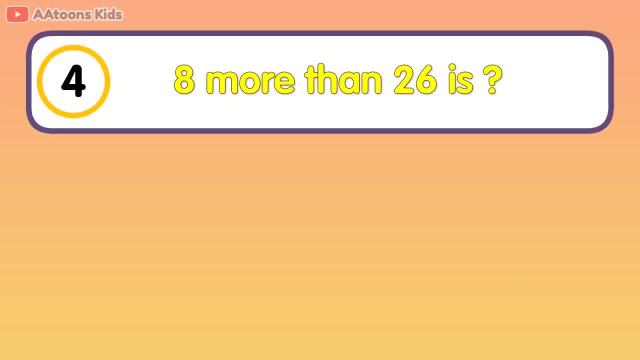 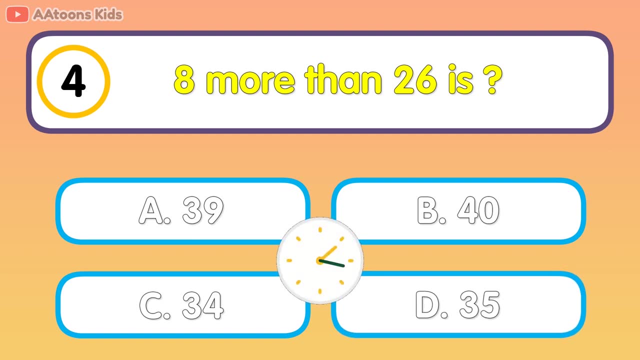 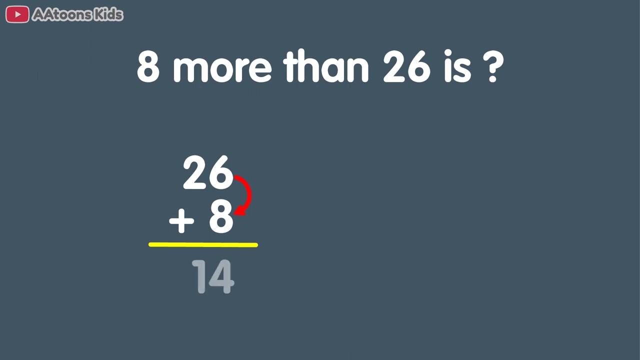 8 more than 26 is 8 more than 26 is 34.. If you add 8 in 26,, it becomes 34.. 6 plus 8 is 14.. Write 4 and take 1 carry. 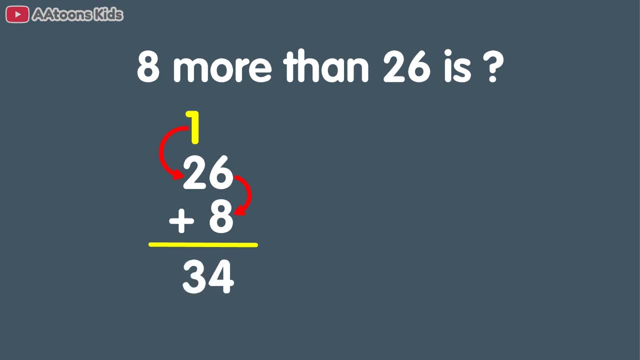 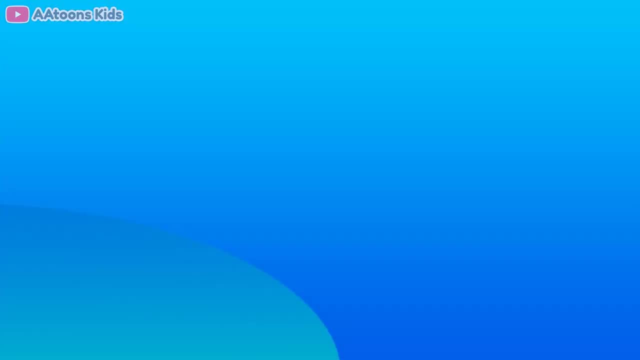 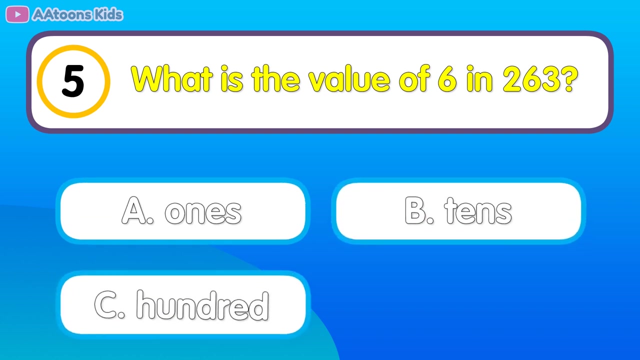 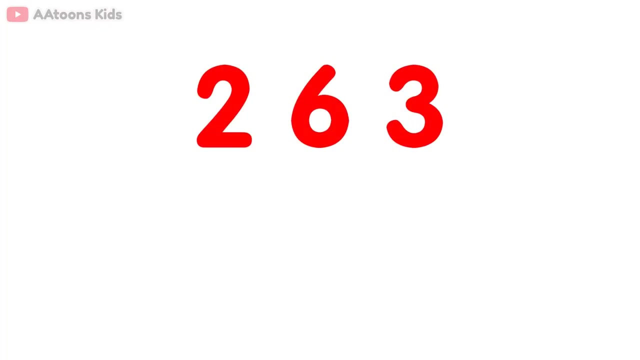 Now, 2 plus carry 1 is 3.. So finally, answer is 34.. What is the value of 6 in 263? 10s? First put the values of numbers 263.. The digit 3 is in the ones place. Its value is 3.. 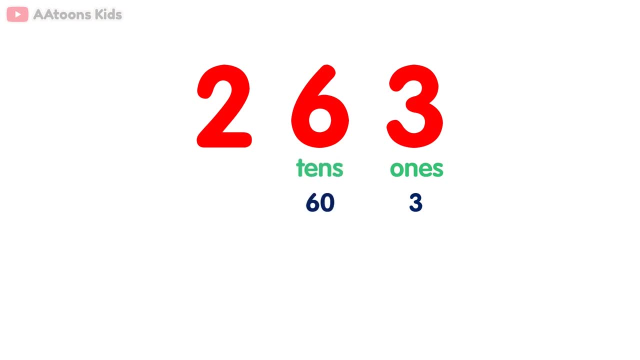 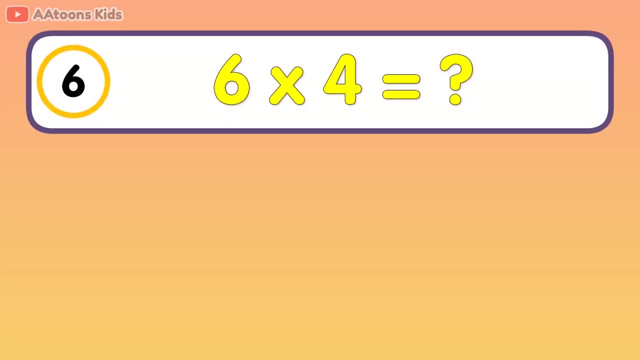 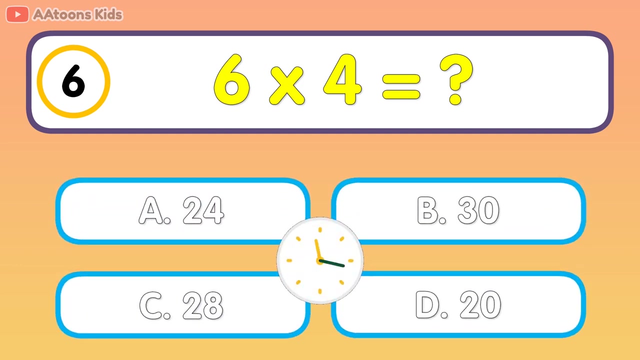 The digit 6 is in the tens place. Its value is 60.. And the digit 2 is in hundreds place. Its value is 200.. So the digit 6 is in the tens place 10s. What is 6 multiplied by 4?? 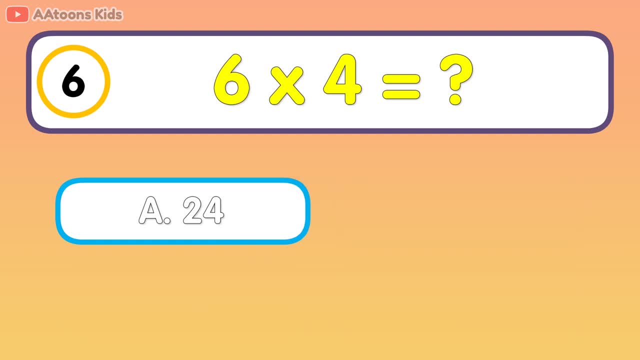 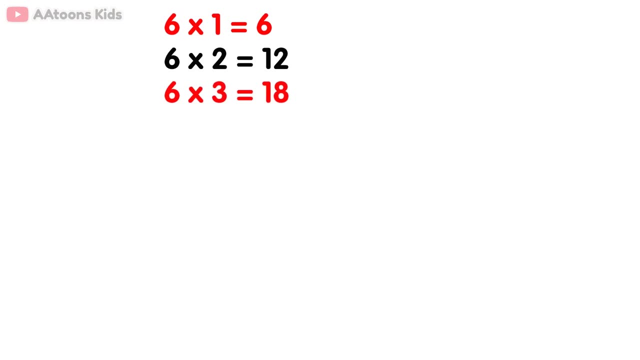 24. First you need to learn multiplication table. Let's count: 6 x 1 is 6.. 6 x 2 is 12.. 6 x 3 is 18.. 6 x 4 is 24.. So the answer is 24.. 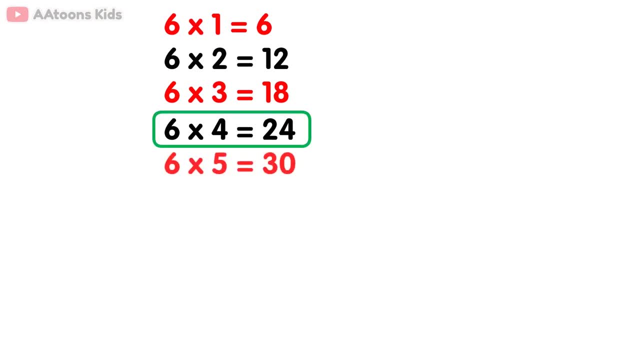 6 x 5 is 30.. 6 x 6 is 36.. 6 x 7 is 42.. 6 x 8 is 48.. 6 x 9 is 54.. 6 x 10 is 60.. 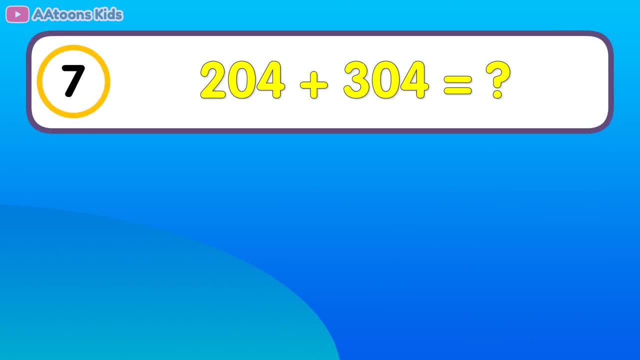 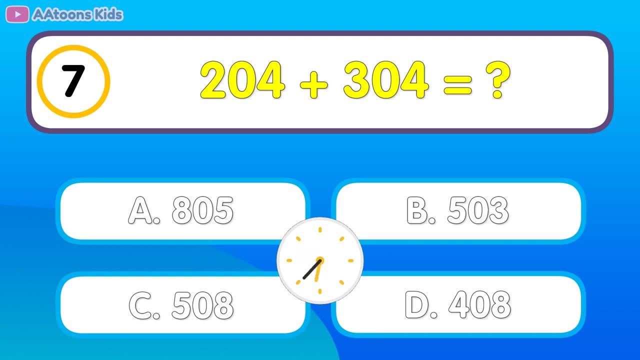 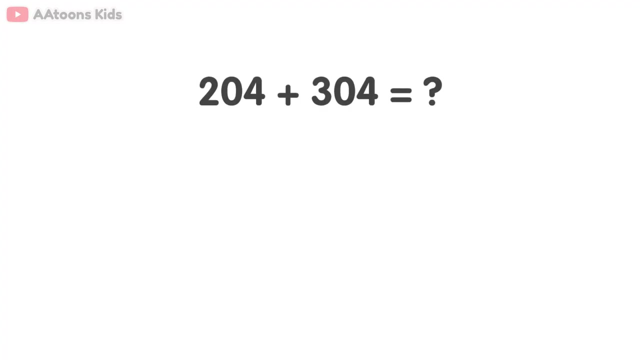 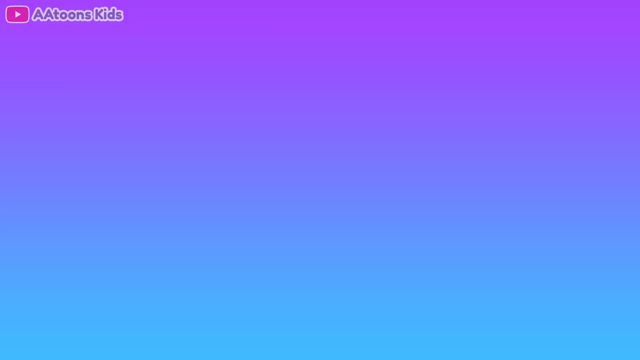 4 plus 304 is equal to 508.. Let's add 204 plus 304.. 4 plus 4 is 8.. 0 plus 0 is 0.. 2 plus 3 is 5.. So 204 plus 304 is 508.. 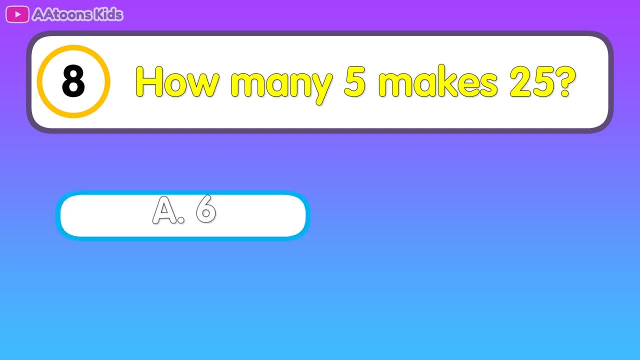 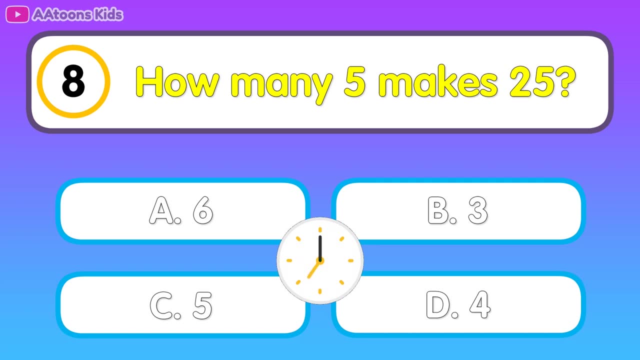 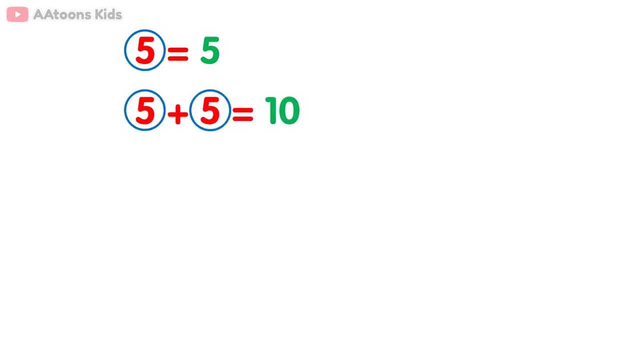 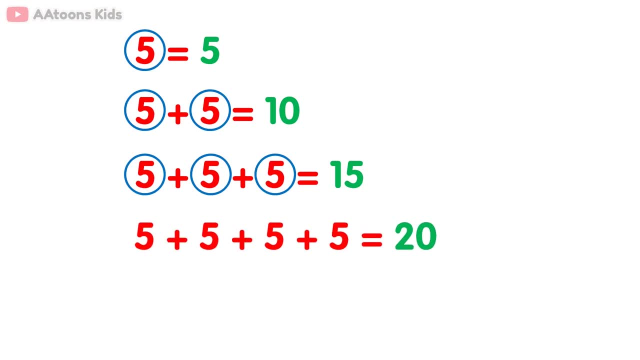 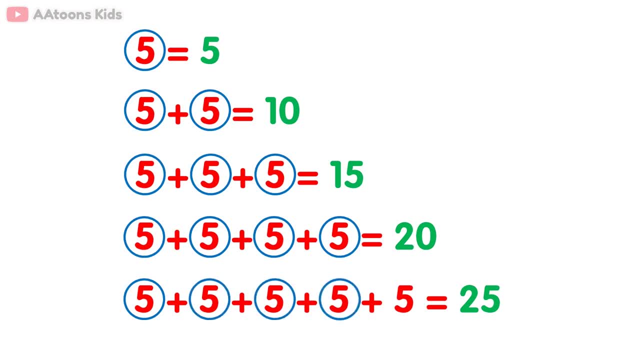 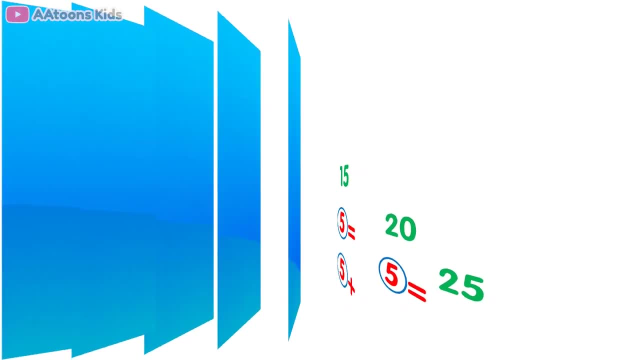 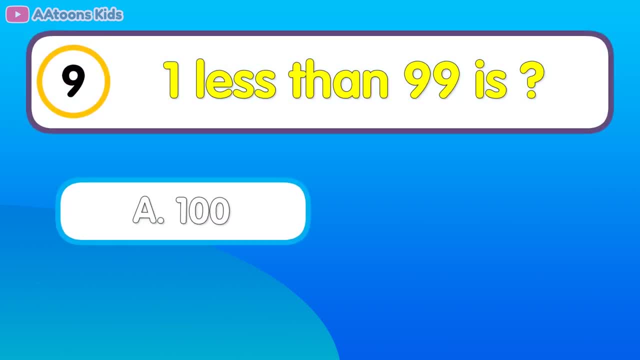 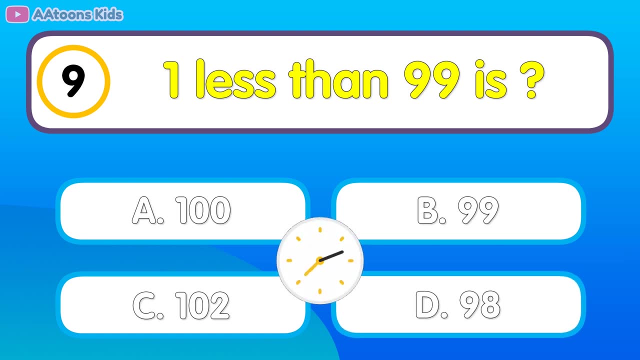 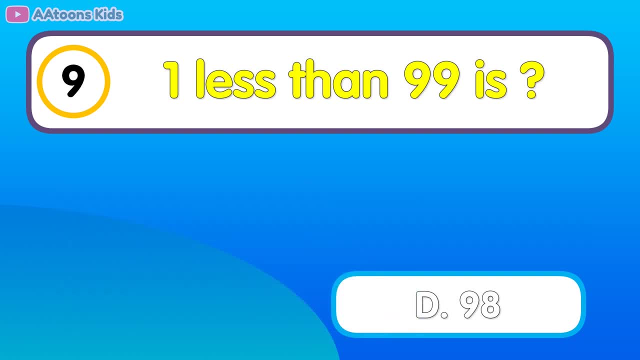 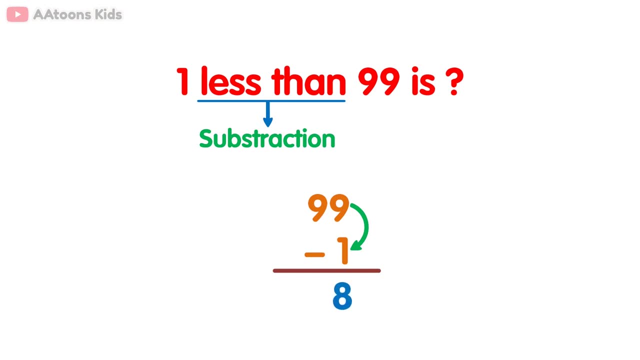 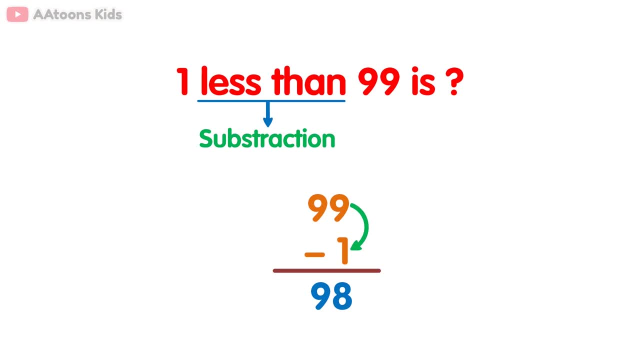 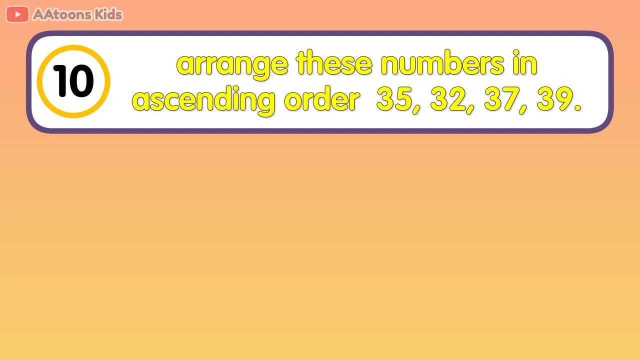 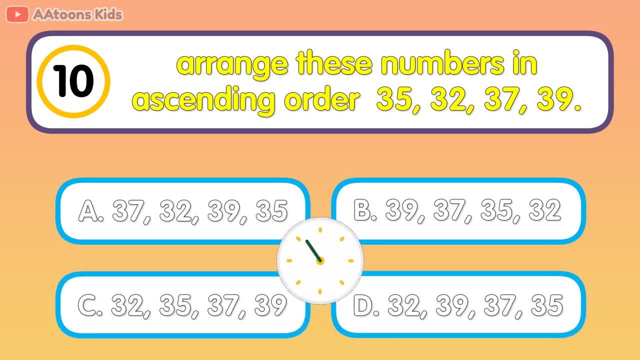 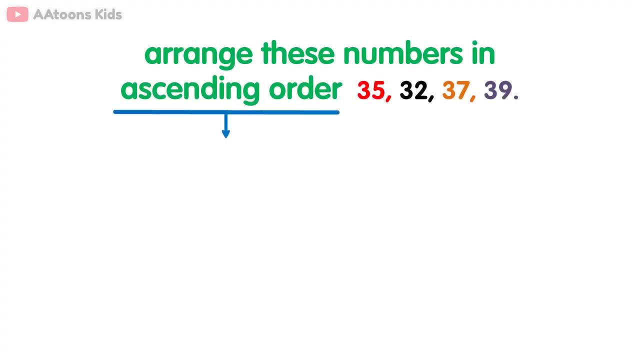 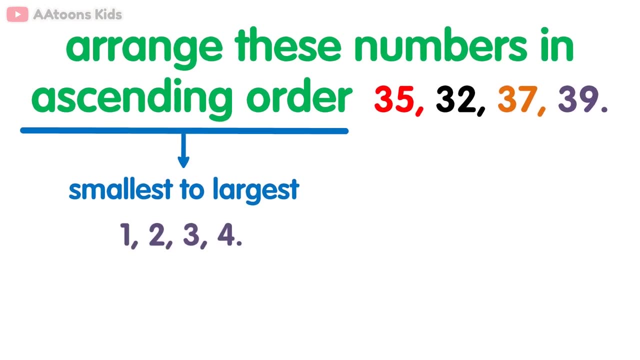 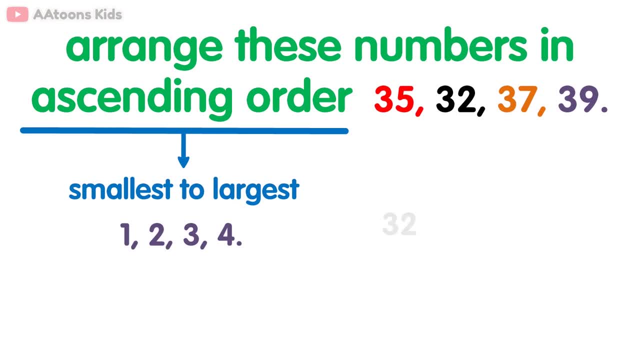 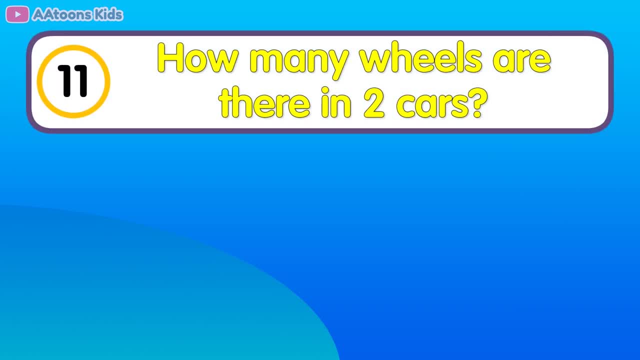 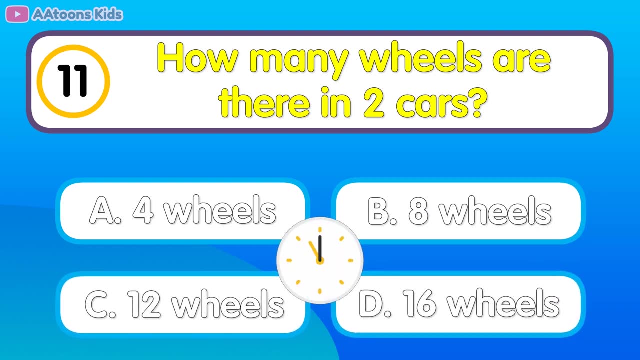 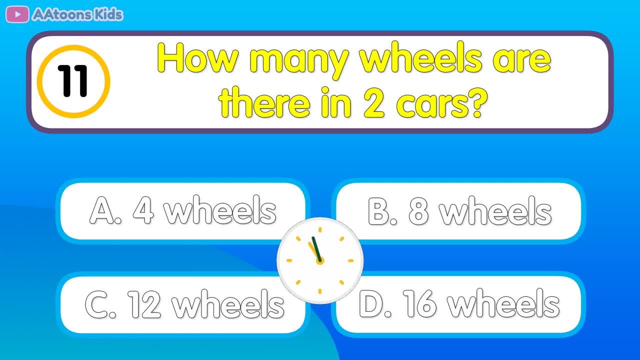 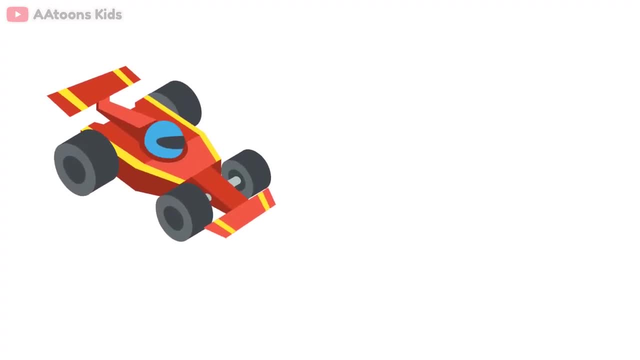 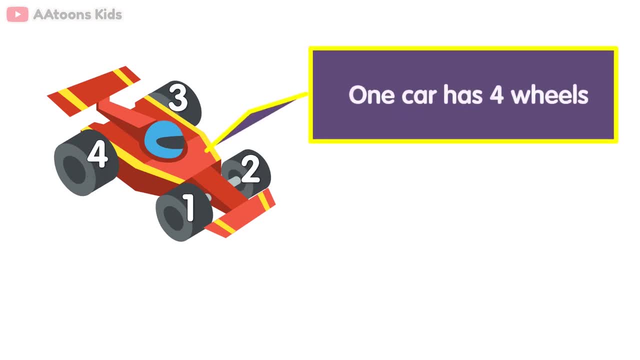 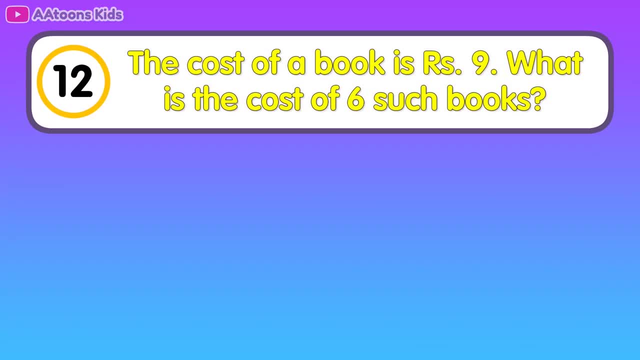 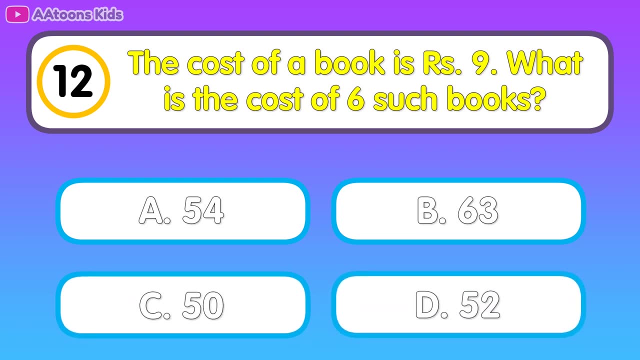 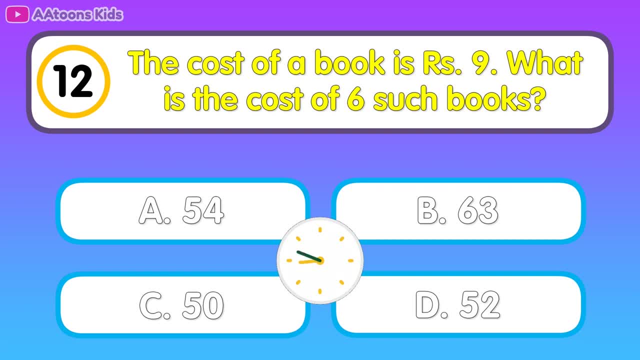 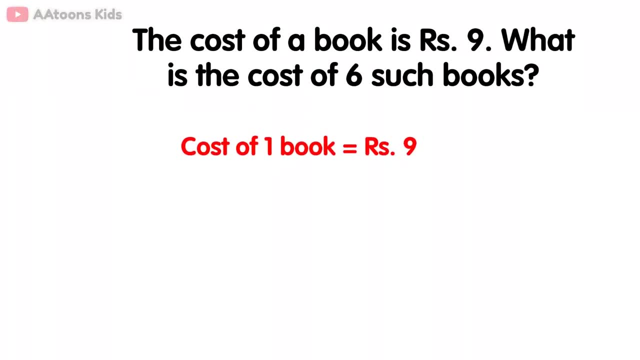 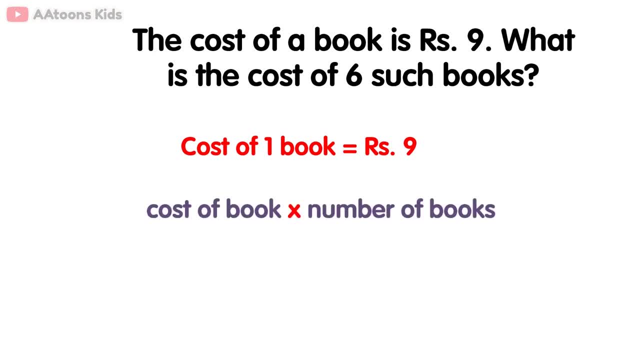 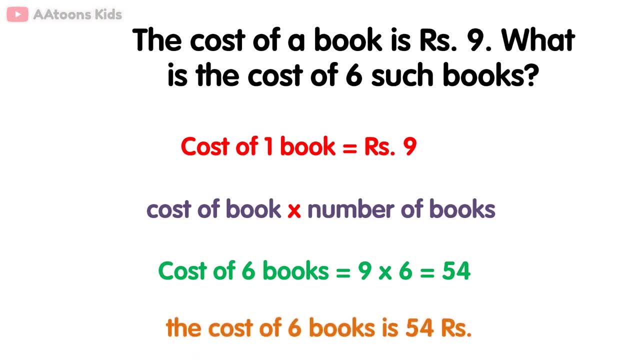 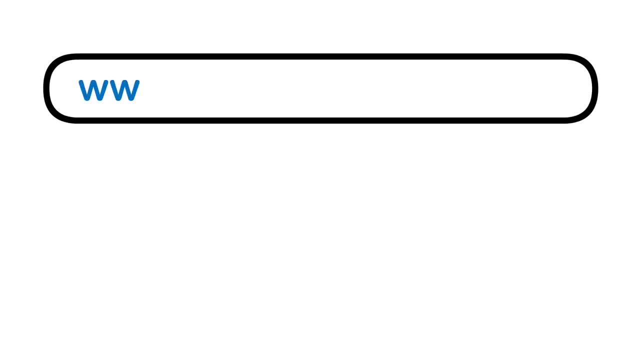